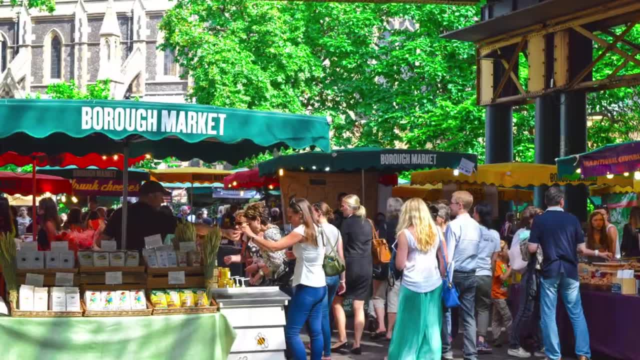 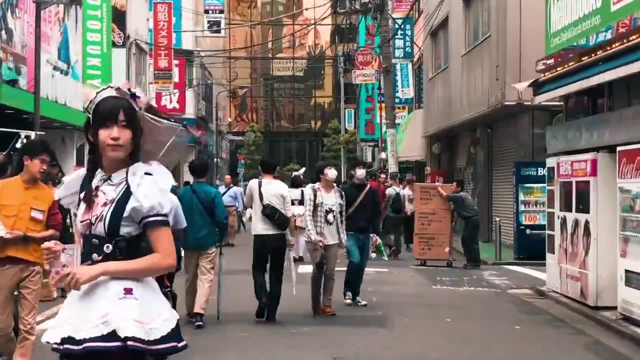 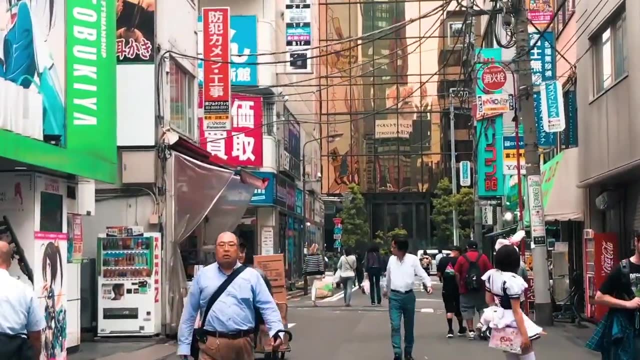 in economics, and that is the market economy. In this type of economy, many individuals make independent production decisions in a free marketplace. It is also known as free enterprise and follows the supply and demand system. Remember not to confuse the market economy with different types of markets, such as perfect competition, monopolies or oligopolies as they're. 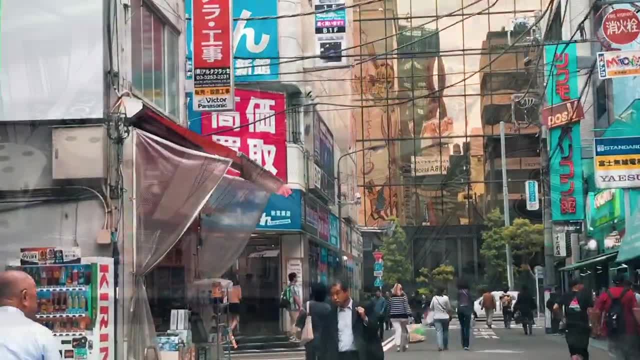 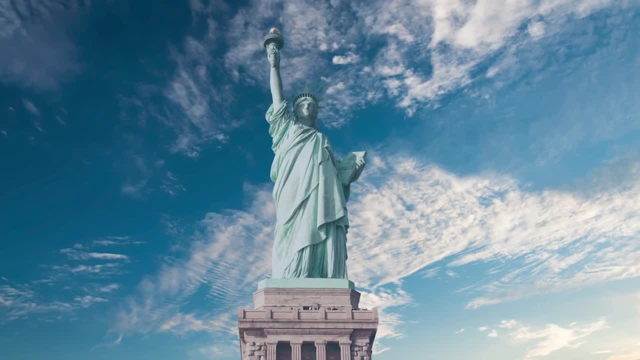 not quite the same thing. In the future, we will upload videos on each of these market types and the implications that each of them have on supply and demand. A real life example of the market economy is the United States, though they could technically be classified under the final. 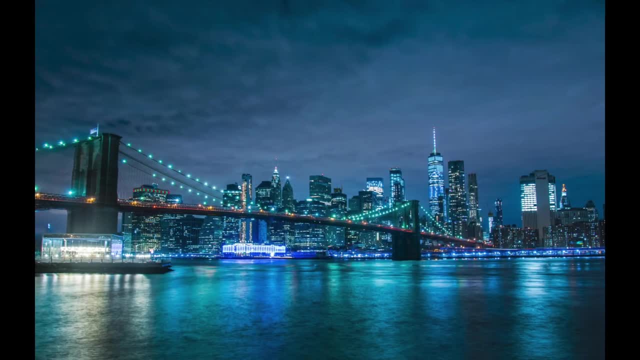 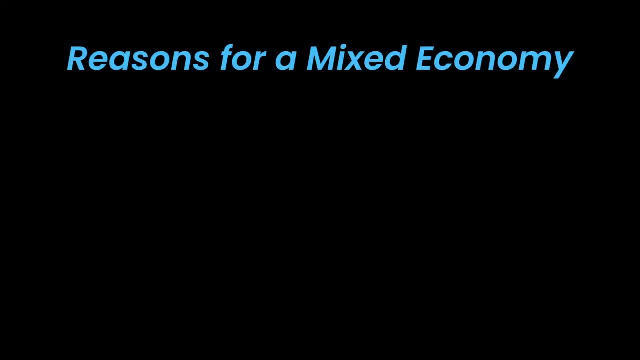 economy type as well. Speaking of which, the fourth and final economy type that you learn about in economics is called a mixed economy. As you may have inferred, very few pure economic systems exist today, for two reasons. One, no single economic system is objectively the best. 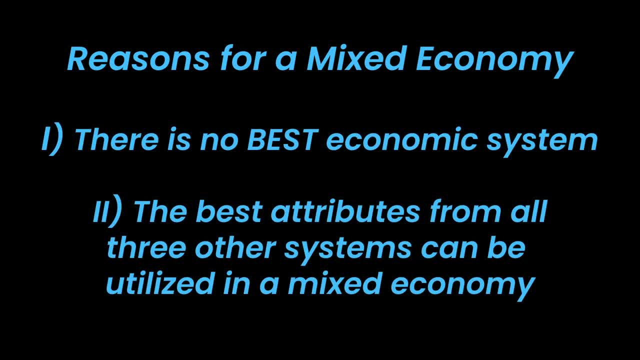 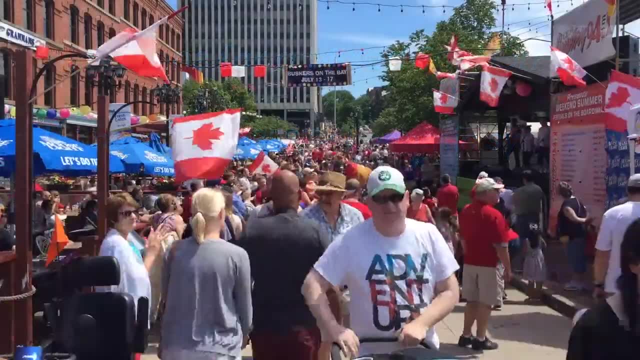 and therefore number two. economic decision makers try to integrate the best elements of each other type into their own unique system. An example of a mixed economy is Canada. The Canadian economy tries to integrate the best features of all three other types of economic systems. It allows for. 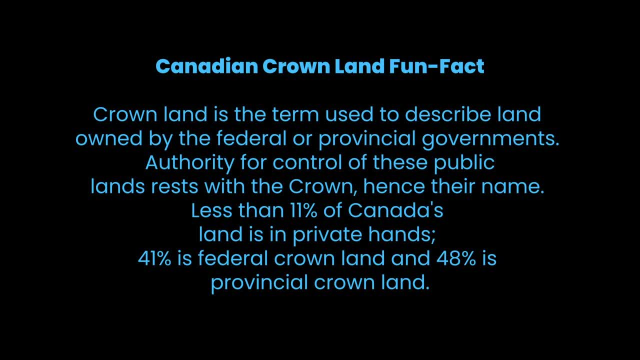 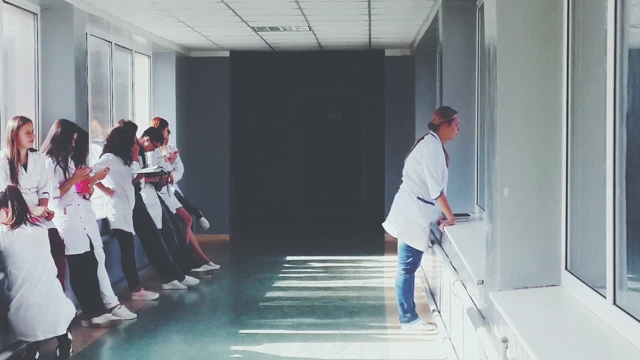 state-owned or crown land, which represents elements of the command economy, but it also allows land to be controlled, which represents market economy. Canada offers many government-run social programs- again a feature of the command economy, but it also has plenty of free enterprise in other areas which. 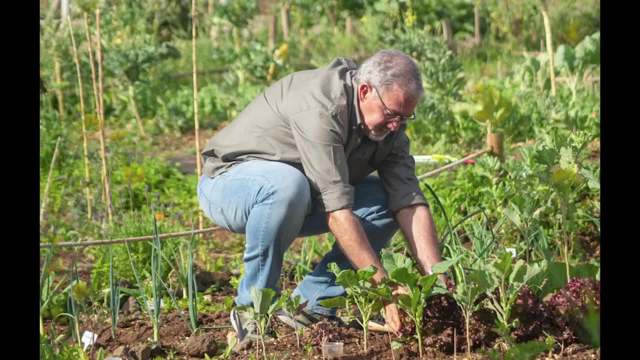 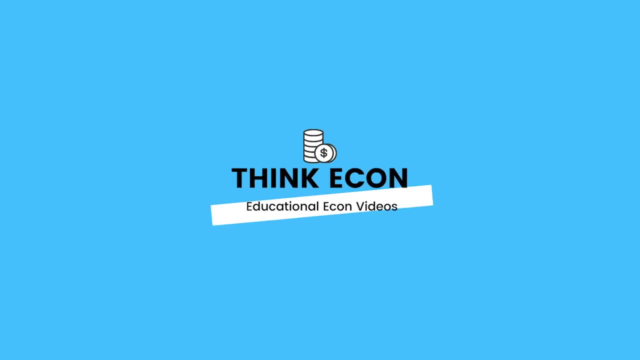 is market economy. Growing your own food and bartering is also becoming a growing practice in Canada, which demonstrates the traditional economy as well. So there we go. now you're familiar with the four types of economies that you learn about in introductory economics. If you like this video and are excited to see more, let us know by liking the video. 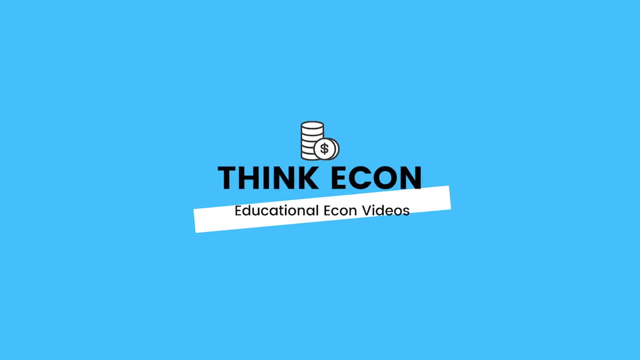 subscribing to the channel and comment what sort of economy you would like to see in the future. As mentioned earlier, we are very grateful for all of the support you've shown so far and it really encourages us to continue producing educational econ content. Thanks for watching this video and 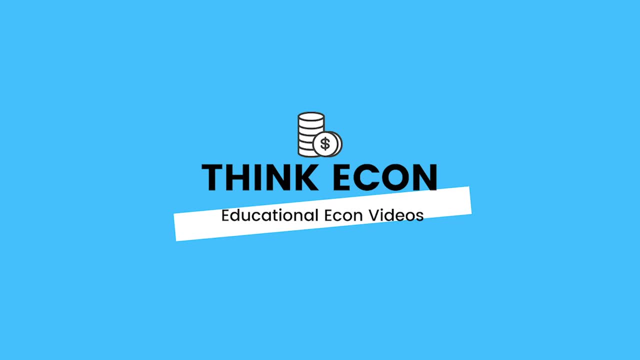 we'll catch you in the next. Thank you for watching.